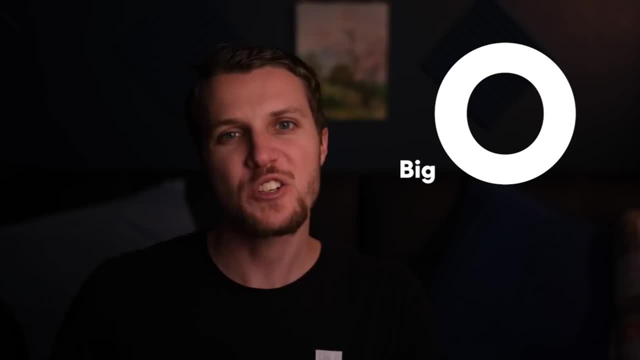 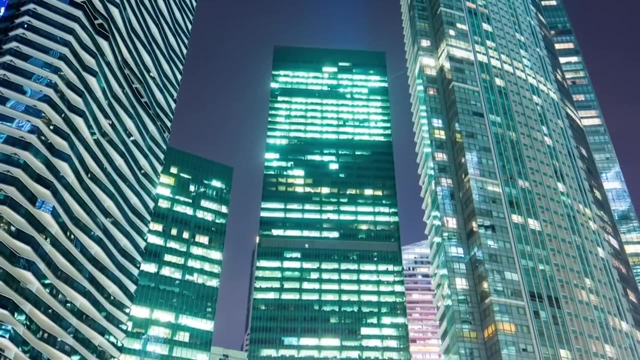 is called the big O notation. This is pretty much a measure of how well an operation scales. So if you have 10 items and then you add a million more, how much longer will each should take? Okay, let's talk about the first data structure, which is the linked list. 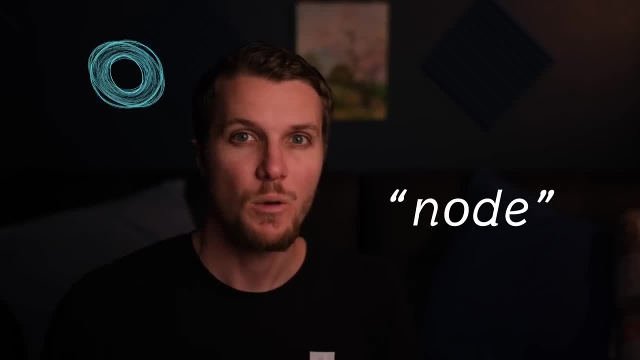 The atomic unit of the linked list is something called a node, which contains a value and a pointer. The value is something as simple as a number like 12, and that pointer will simply connect you to the next node in the chain. hence the linked part of linked list, The first node in 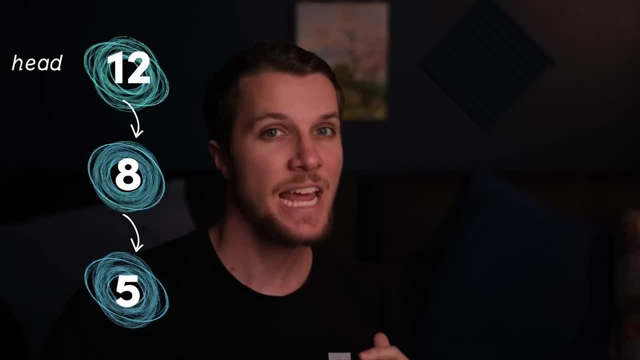 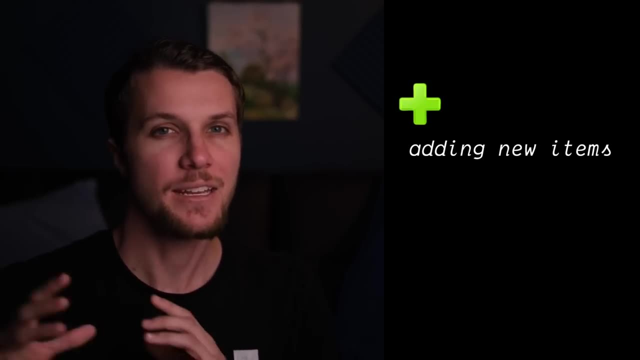 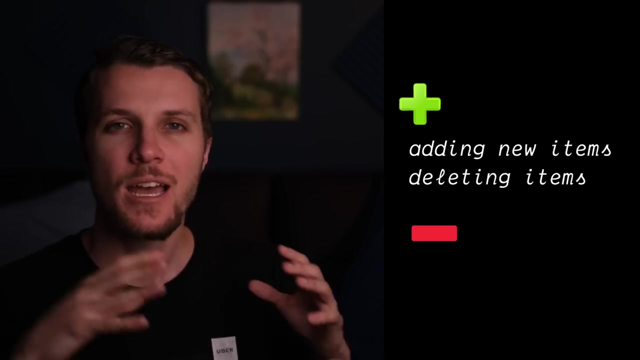 the list is known as the head, while the last one that doesn't have a next pointer is known as the tail. Pros and cons of the linked list. It's really good at adding new nodes and deleting nodes, because we can just change where the next pointer is pointing. However, it's not too good at retrieving. 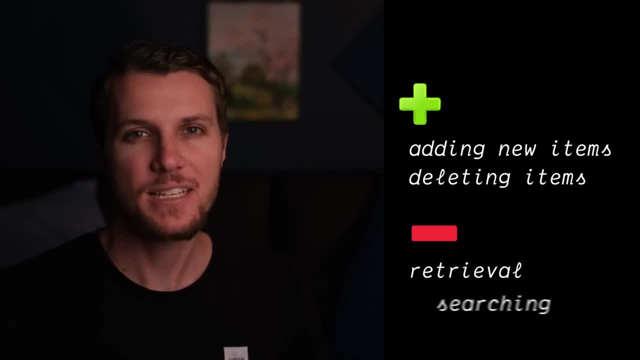 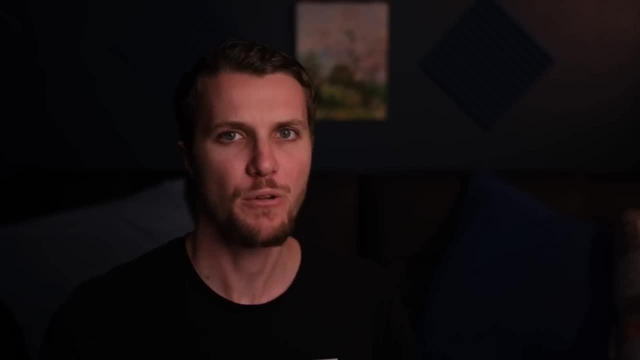 nodes, even when we know the index or searching, because each node is only aware of the node next to it. Data structure number two is going to be the array. You might already be familiar with arrays because they're super common in all programming languages. The array is quite 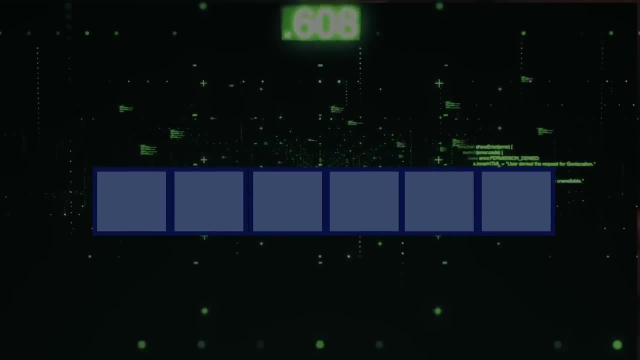 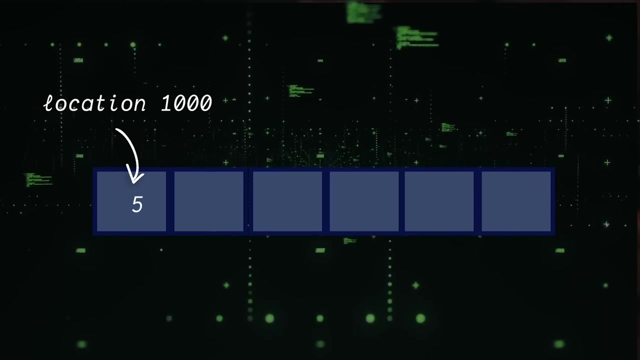 literally a continuous block of cells in the computer memory. By keeping track of its memory location. let's say the location is 1000, it can instantly compute the location of any item inside of it. For example, let's say we want to get index number five. We just add five to a. 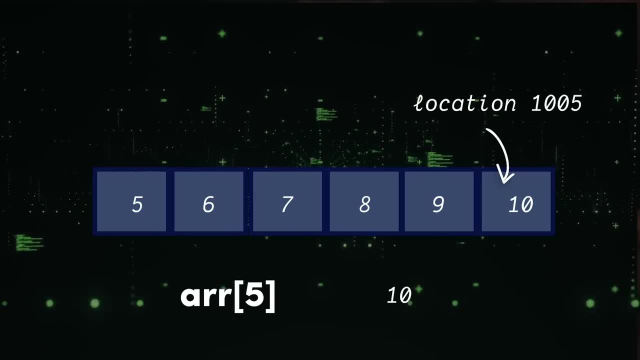 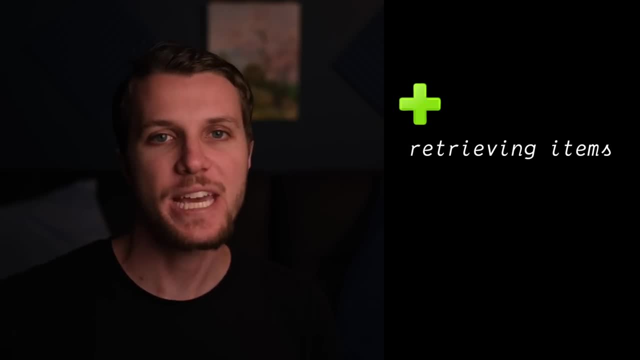 thousand, get a thousand and five, and then we can pull that value directly out. As a result of this, you can probably imagine arrays are really good at retrieving items. However, consider this: your array keeps growing in size and you start running into other things in memory. 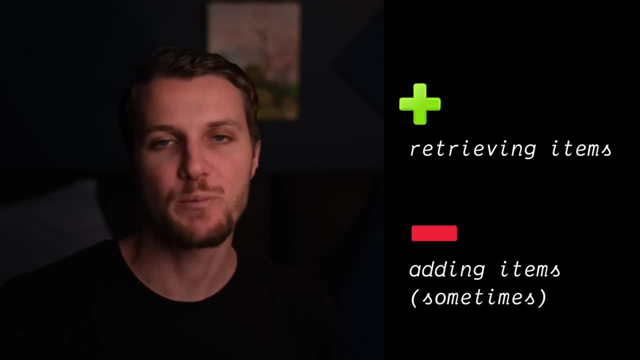 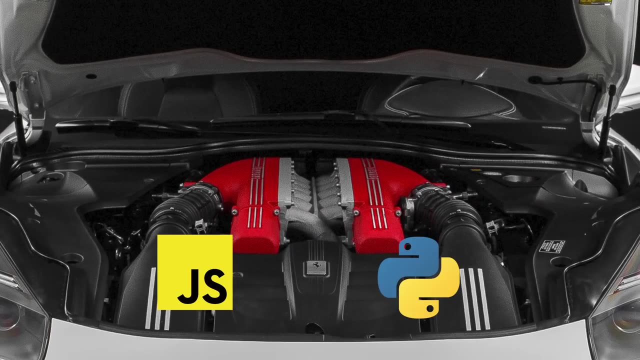 For this reason, adding isn't always too efficient, because we might have to move our array to a new place so it fits. Luckily, this happens under the hood in high level languages like JavaScript and Python, but in lower level languages you have to declare the. 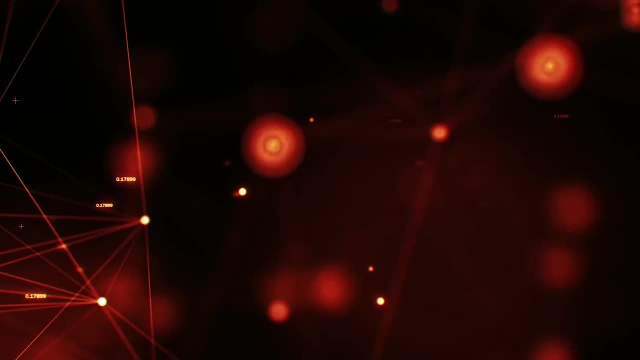 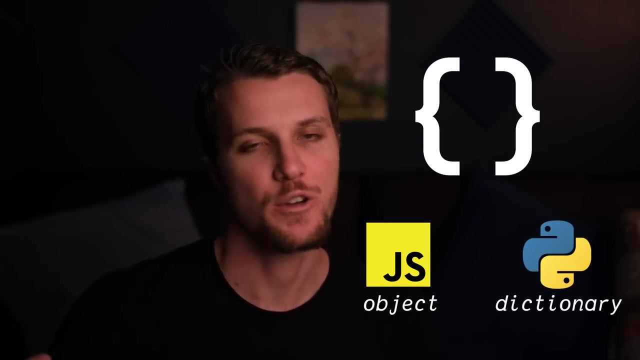 size of your array in advance. Okay, the third data structure in this one is super important- is known as the hash table. You might be familiar with it because it's an object in JavaScript or a dict or dictionary in Python. I think dictionary is a great word because you basically give the 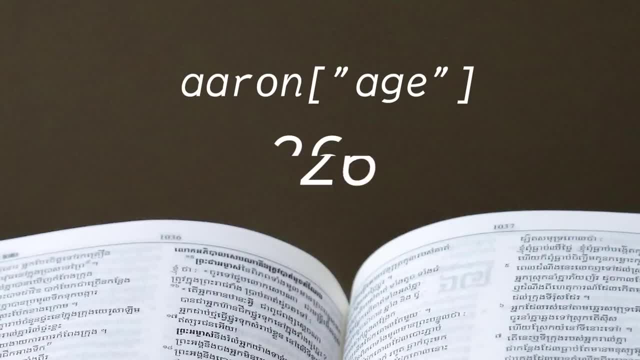 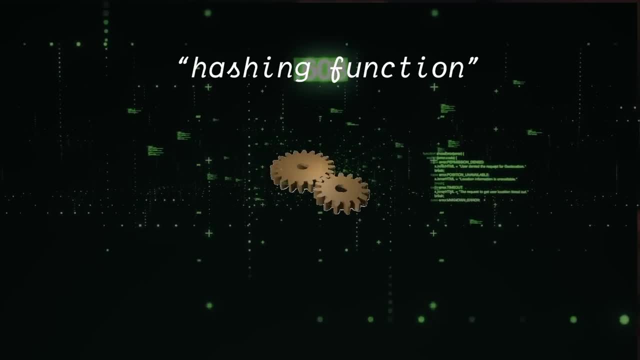 hash table a word or a key and it will retrieve the definition or the value for you On your own. it's a lot like an array. The key actually gets run through a function called the hashing function and that will spit out a memory location for you. The way it's different is these memory. 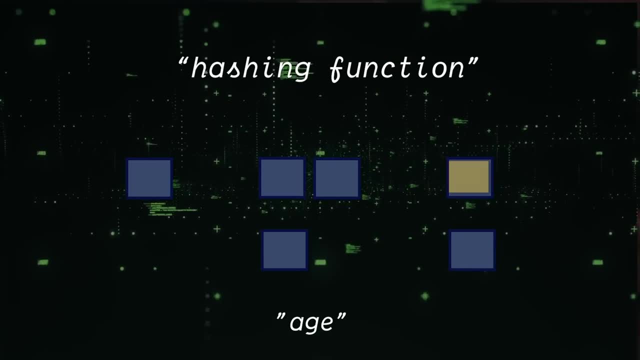 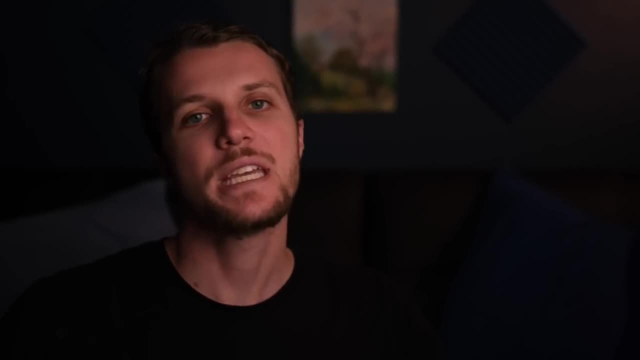 locations don't have to be next to each other. They can be anywhere, So you don't have the same problem with the increasing size. However, there is a different problem Depending on the hashing algorithm you use. two keys could hash to the same memory location. This is what's known as a 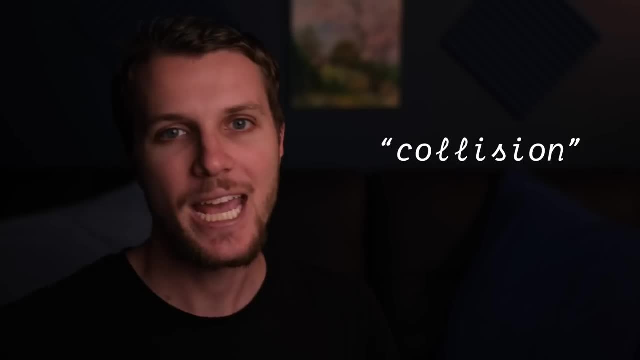 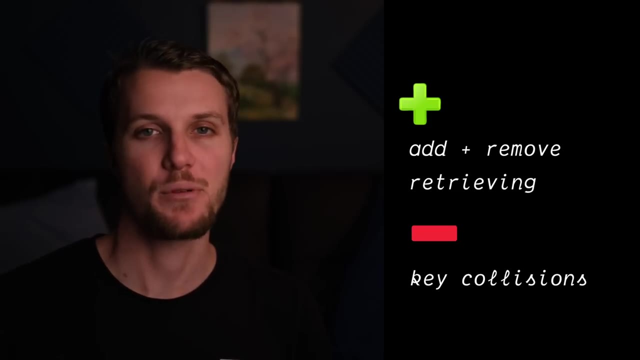 collision and there are different ways to resolve this, but again it's all happening under the hood. The hash table is really good at both retrieving and adding, but the collisions can be a problem. Okay, fourth, data structure. this is a double: is the stack and the queue. 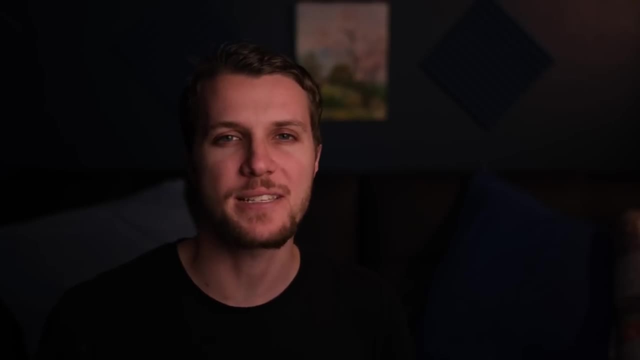 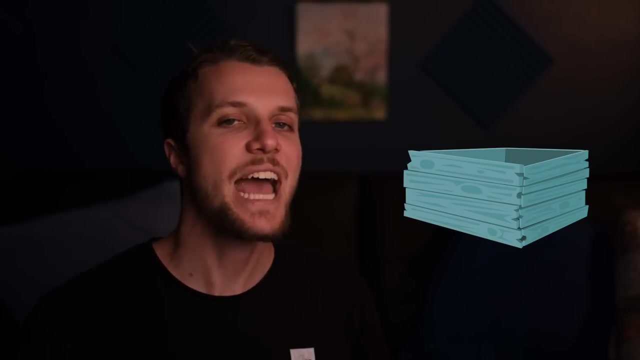 I'm grouping them together because they're pretty similar and they're both kind of built on top of arrays with a few additional features. The stack is a last in, first out data structure. Think of a stack of cafeteria trays: The last one you put on the top is the first one you have. 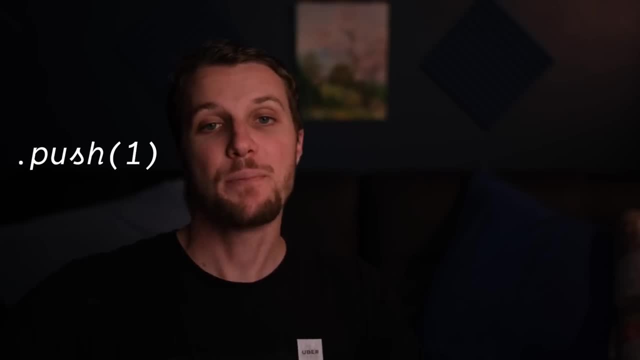 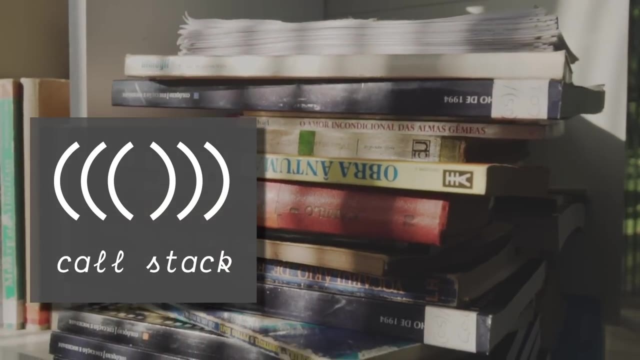 to take off When we add an item to the top. it's called pushing, and then we pop off the top. Every language keeps track of the functions that have been called with something called the call stack. Stacks are also super important for an algorithm called depth first search, which you're. 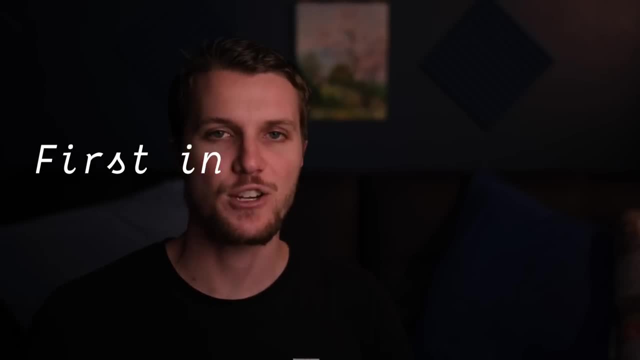 going to run into a lot. The queue, on the other hand, is first in, first out, just like any queue or line, Let's say a line to board a plane at the airport. Adding an item to the end is called in queuing and removing it from the front is dequeuing. Queues are used for a really important 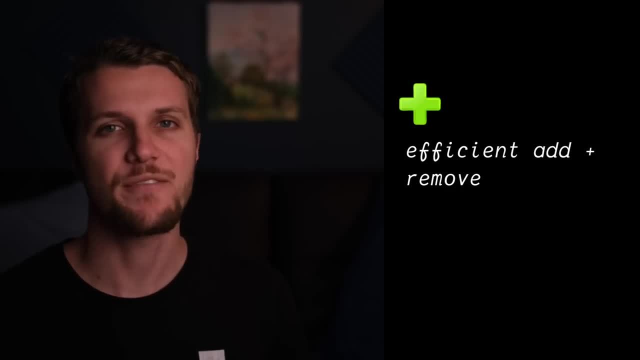 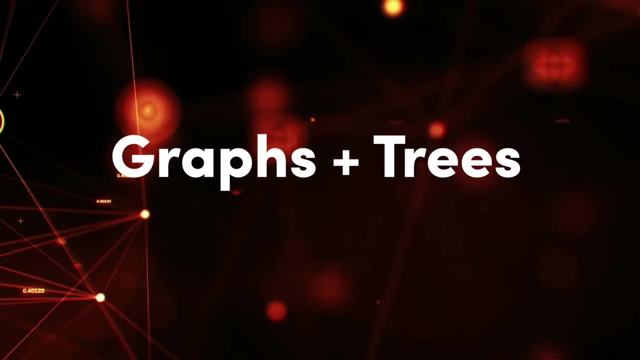 algorithm called breadth first search, Overall stacks and queues are really efficient, but at a limited use cases compared to other data structures. Finally, we're going to talk about graphs and trees. This one is so big that there's an entire field of computer science called graph. 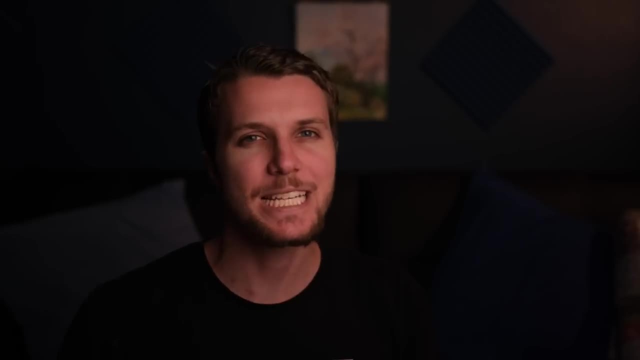 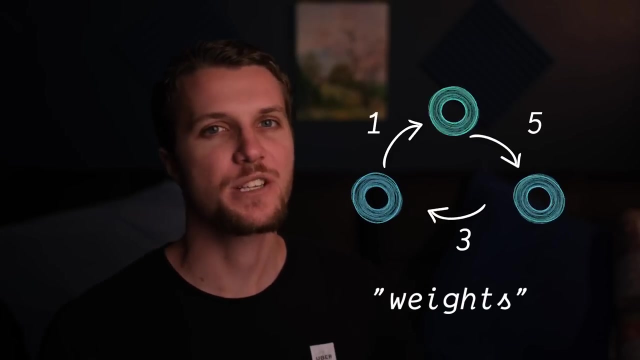 theory. What a graph is is basically kind of similar to a linked list where you have nodes that are pointing to other nodes, except in this case the pointers are called edges. Edges can also have weights or numbers assigned to them. Imagine two cities, New York and Boston. The road: